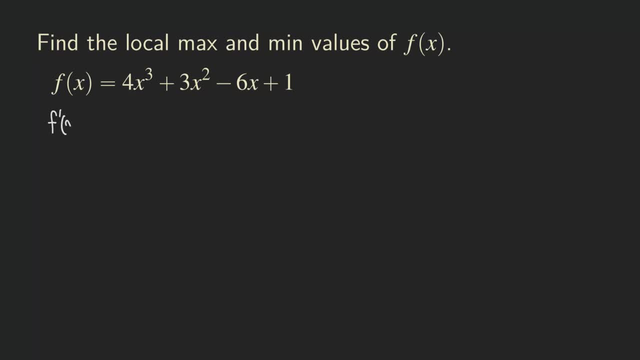 function. So we have f prime of x. okay, that's equal to 12 x square, and then plus 6 x and then minus 6.. Okay, so that's our derivative. And then, when we need to find the critical numbers, 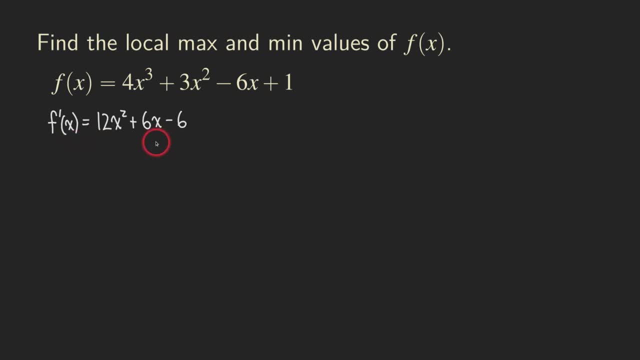 and for the critical numbers we need to. we have two cases: either f prime is equal to zero, or f prime does not exist, And so for the case when f prime is equal to zero, then let's just start writing down this information here. we need to find the critical numbers. Okay so, 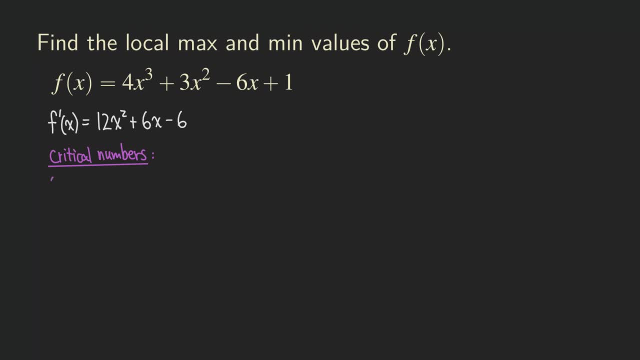 first case is that f prime is equal to zero. Then in this case, what are we going to be getting here? So that means that 12 x square, we can set this derivative, the first derivative, equal to zero, and then we try to solve this equation, And so we can factor out six from all the terms. 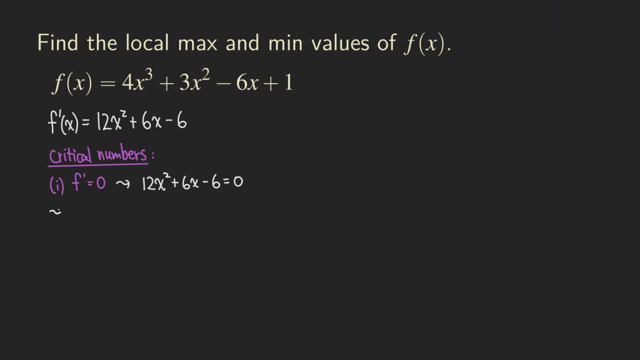 then we are going to, we are going to get what we are going to get- six- and then we are having two x square and then plus x and then minus one, and that's equal to zero. And then now we can factor this: two x square plus x, minus one, So to factor that we are going 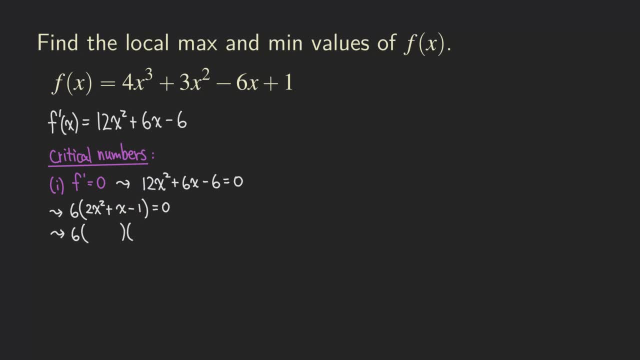 to get six and then times. Now we will factor this trinomial as a product of two binomials, right? So first we need to come up with two terms that will multiply to two x square, And so that would be. that would be just x, right? So let me put down the x right here. 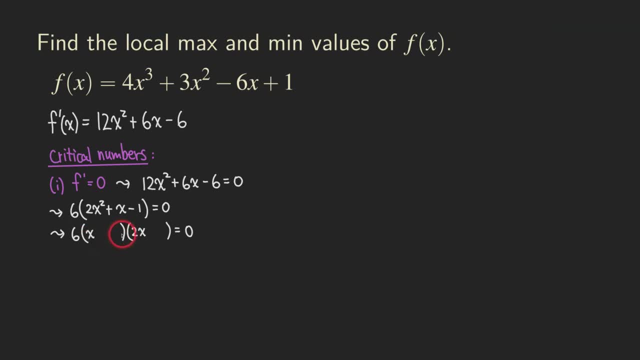 x and then two x, And then we also need to figure out two numbers. when we multiply them, we are going to get the one. So we are going to get the one here and then the one here. So one times one will give you the one. And then now we need to worry about the signs, Because we are 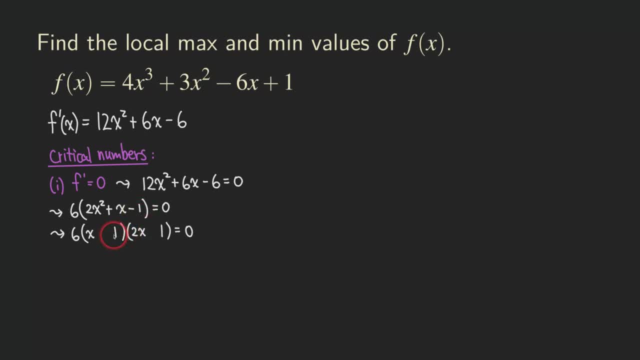 having a negative one right here. So that means one of the ones has a positive, has a positive sign, and then the other one will have a negative sign in front of it. Okay, so now let's check. If we look at the middle turn, the middle turn has a positive one x, And to get positive one x, 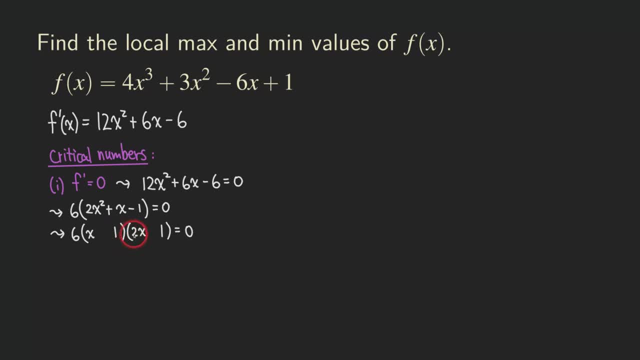 we actually need to get the this one times a two x to be a positive, positive two x so that we can get the positive x. And so what we are going to do is that we are going to put a plus sign in front of this one right here, And then we are going to get a. 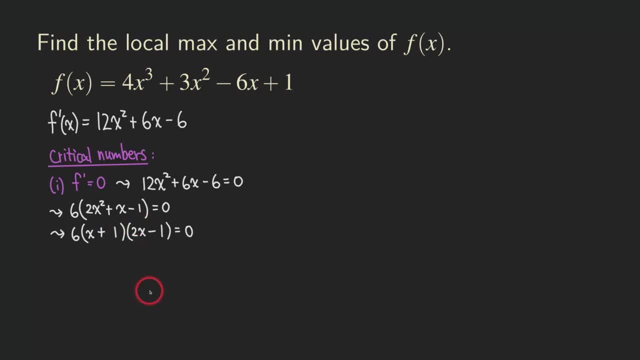 put a negative sign here, Okay, And then we can do a quick check. we have two x And then that's negative x, So that will give us the positive x. So now that's good, And so if we are solving this equation, then we are going to get x equals negative one here, And then the 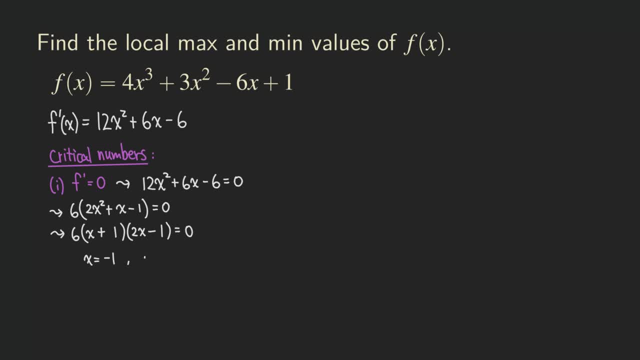 other possibility is that x is equal to one over two. right one over two. when we substitute into this x- right here, we get two times one over two, which is 11 minus one. we get zero. Okay, so those are the two solutions for this equation, And so that means okay, if we do the this one. 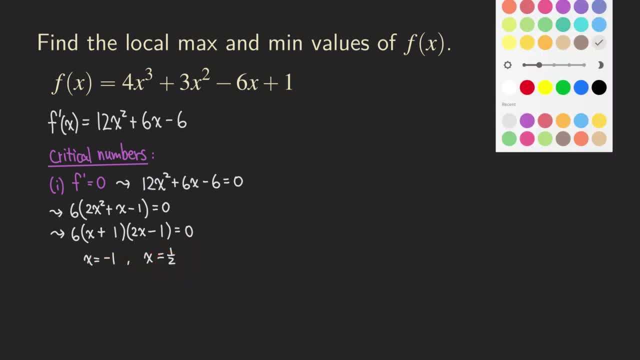 those two are the critical numbers. And what about the other case? The other case for the critical numbers, for finding the critical numbers, is that f prime does not exist. Okay, but because this is a polynomial, so we cannot really find any values for which f prime. 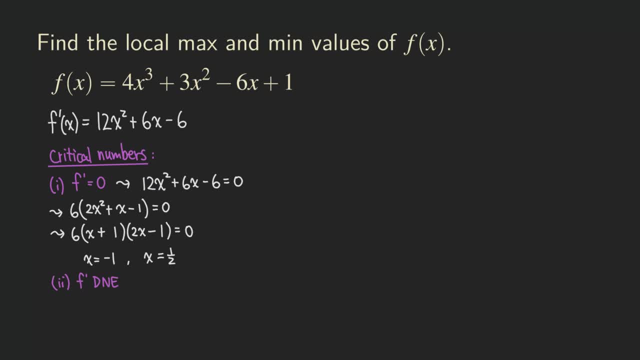 does not exist, And so that means we are not going to be getting any values right here. So there is no value for this subcase here. no values. Okay, so we have our two critical numbers, So next step is that we are going to make a sign analysis chart so that we can use the 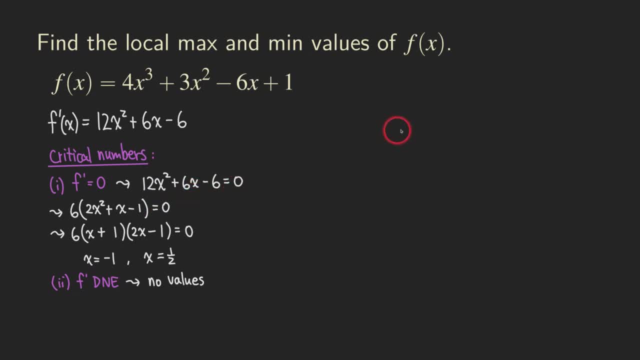 we can use that. what is that? the first derivative test. Okay, so how do we do that? We are going to first start by drawing a lumber line here. So let's do that. So let's draw a lumber line. Okay, let's draw this lumber line right here, And then this is actually our x-axis. 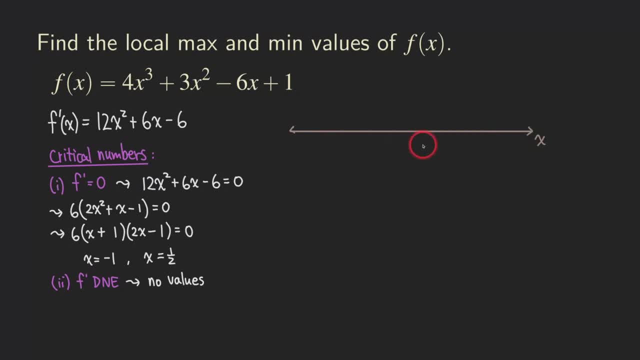 Okay, and then we can just do some labelings on there. What do we need to label on this lumber line? For this lumber line, all we need to label is that- the two critical numbers on there. We do not need to label any of the other numbers, So we are getting negative one. 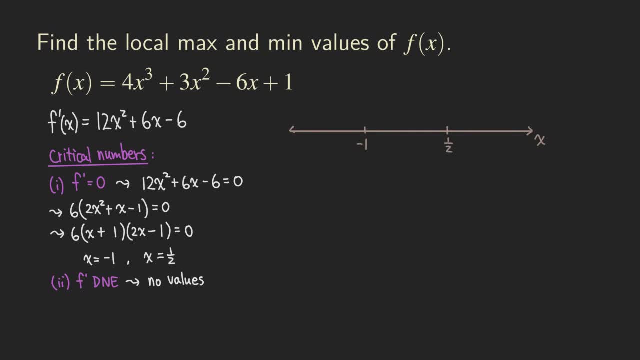 and then the other one is the one over two. Okay so, and those two critical numbers will break the lumber line into three intervals. So there is one interval for all the x values less than negative one, one interval for all the x values between negative one and one over two. 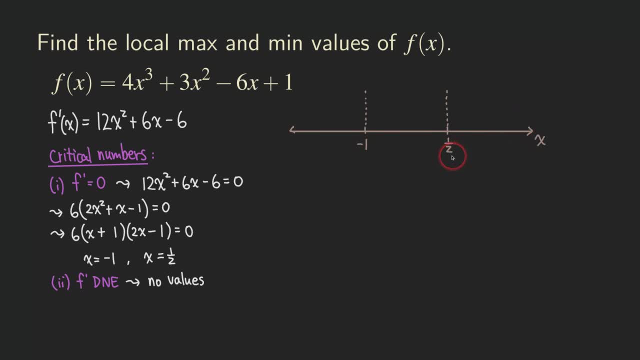 and then all the x values that are greater than one over two. Okay, so now we are going to, we are going to pick a number, So we are going to pick a number and then we are going to plug it back into our derivative and do the checking, And so what we can do is that we can, we can pick, we. 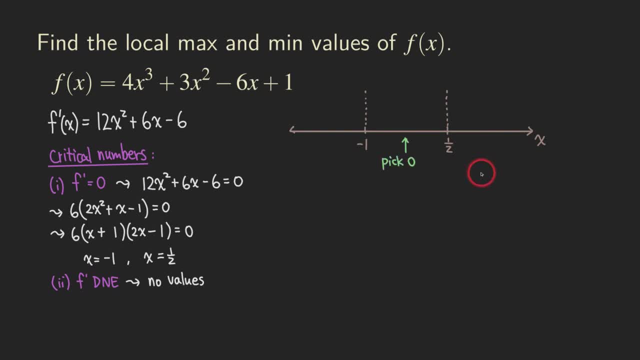 can pick. what can we pick here? we can pick zero, because zero is between a negative number and a positive number. So that's for the ease of the calculation. Actually, it doesn't matter what numbers that you pick. between the negative one and the one half, you can pick point one and point two. 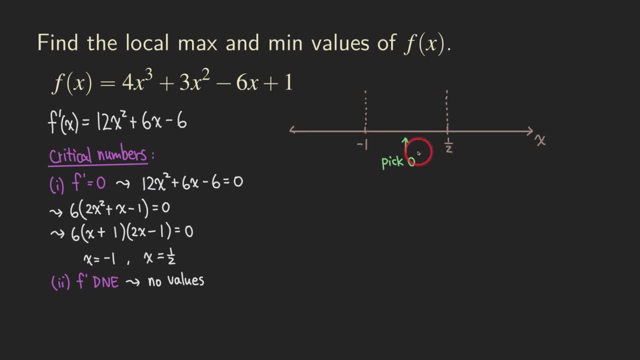 point three: as long as less than one half and greater than negative one, then that will be okay. But usually we just pick an easy number for the purpose of the making the calculation easier. Now for this one we are going to pick, since this is a polynomial, the domain is all real numbers. So 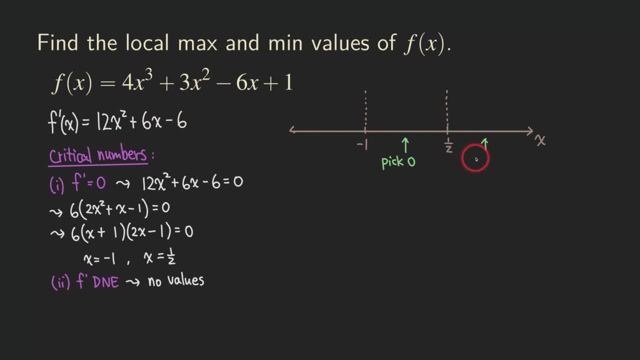 that means we can pick any numbers that we have here, right? And so what we can pick here is that we are going to just pick a large number, we pick 1000.. And then, on the left side of this negative one here, we are going to pick a negative 1000. 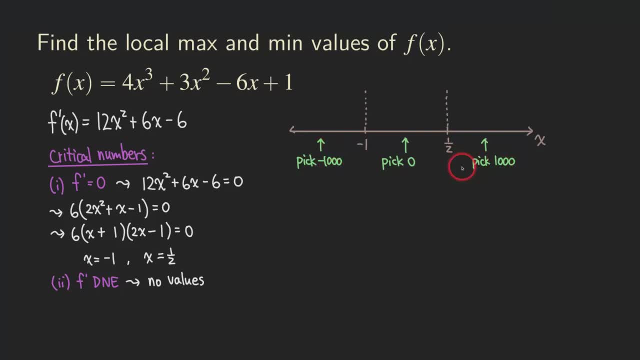 And then you may say: why do I pick those big numbers? You will see in a few seconds why picking those big numbers will be really helpful for checking the signs, because all we care are the signs right. We don't really care about what the answer is when you plug in those numbers into the. 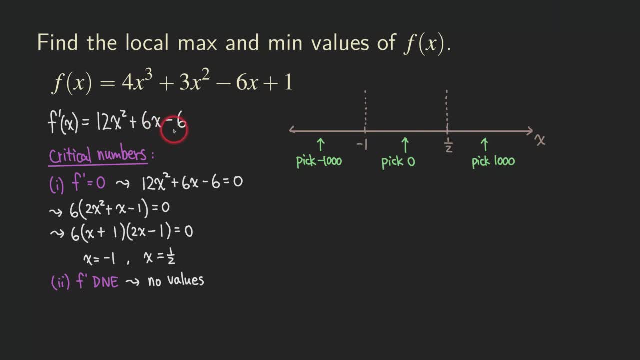 derivative. So now if you plug in the zero in here we can do the calculation really quickly. that's actually just a wide intercept of the first derivative. So that will be negative six, And so that means we have been put a minus sign right here. So that's minus sign. Okay, so that's that. 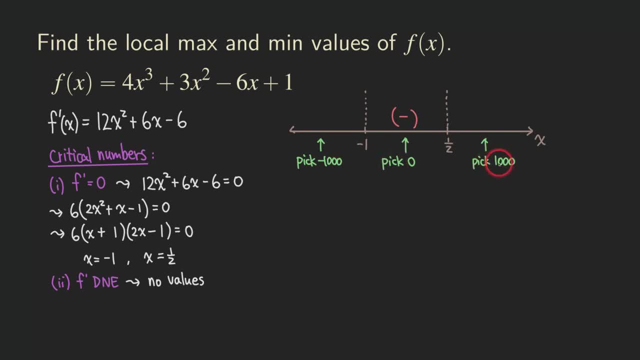 And then the next one. the next one would be what we plug in, the 1000 in there, And, as you can see here, when you're plugging the 1000, it becomes really obvious that the the sign will be positive. even though the negative becomes positive, right? So we want to make sure that, since we'd alreadymel部分 placed to zero for all those of the blank users, we can have an answer now to check the signs. So that's going to be positive. So let's see what we are going to do now. Let's add a number to the Fleur's gets. 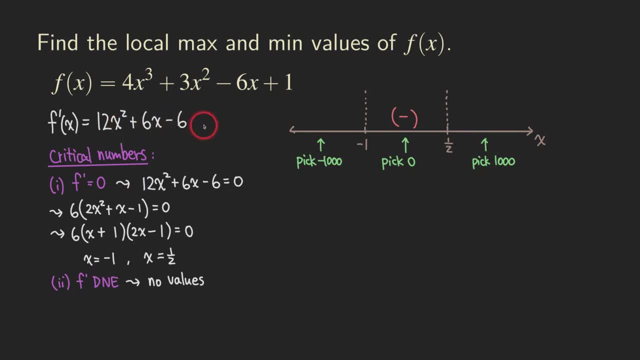 the sign will be positive, even though we don't know what this number is equal to, And so we are going to get positive. And then the same thing here: when you plug in negative 1,000, you are going to score that negative 1,000. 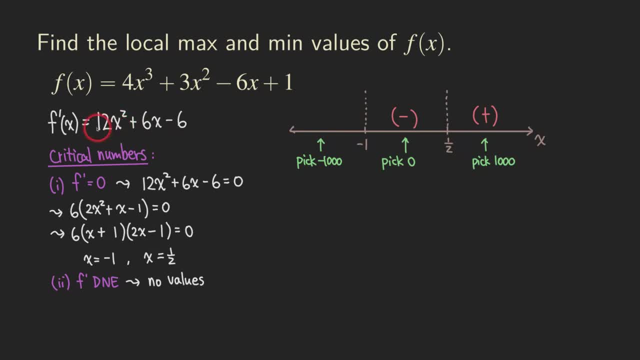 So it will become a million. And then you multiply that by 12. And even though you are going to plug in the negative 1,000 in here, which will give you a turn of negative 6,000, but that's too small compared to your leading turn here, right? 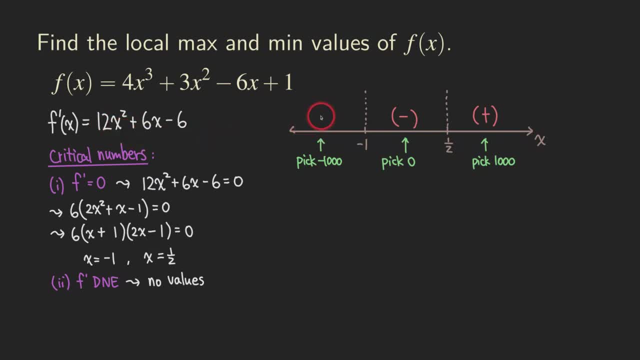 Your dominant turn for this first derivative. So this would still be a positive quantity. And so you may say: why do we care about all the signs? It's really because we let's say: for this interval, the derivative is negative, right? 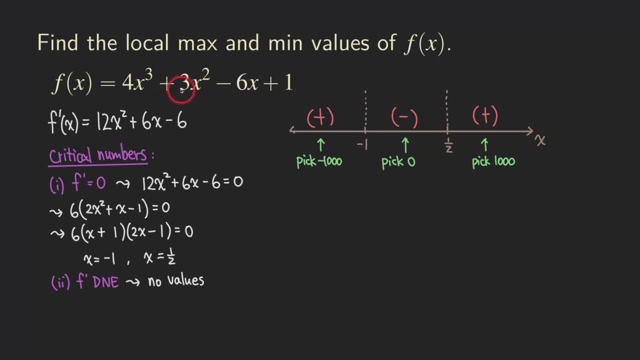 What does that mean? That means the function, the original function, the f, not the f prime is decreasing on this interval. So that means f is decreasing from negative 1 to 1 over 2.. So we can now actually write down the result right here. 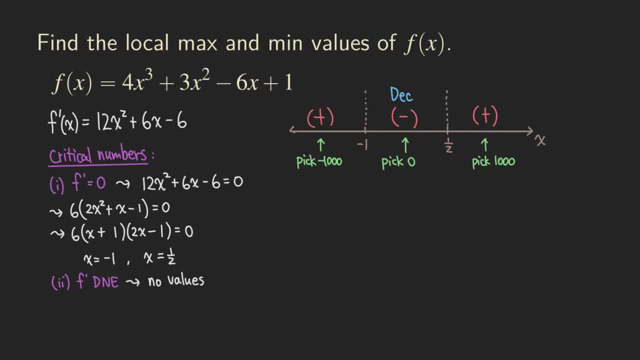 The function is decreasing, Okay, And then for the intervals, that in which the f prime is positive, then the function, the original function, is increasing. So now we can actually write down those information right here. If we are writing down the information, then we are going to. 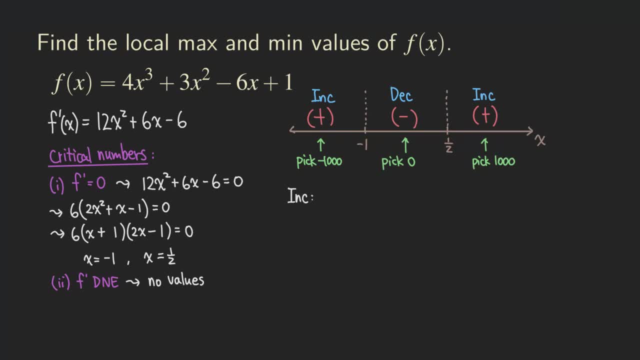 we are going to get what we are going to have this. So the increasing intervals for the function it's going to be first one is from negative infinity to negative one right. So we are going to just put that down right here. So what is that? 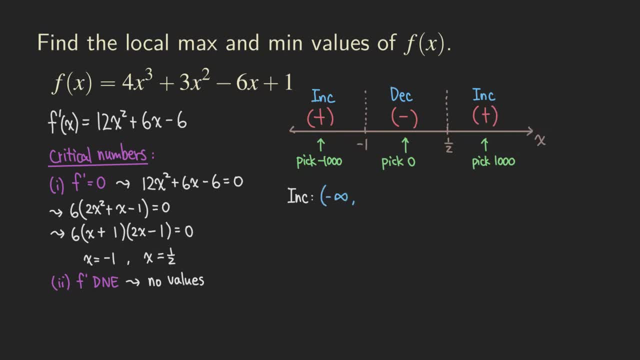 That's. that's like the infinity to negative one. And then what is the other interval? The function is also increasing from one over two to infinity. So we are going to get the second interval, So one half to infinity. Okay, So that's that. 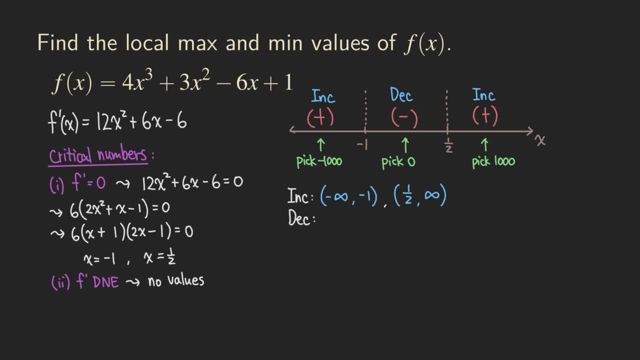 And then we can also write down the decreasing interval right here. What really happened is that there was only one interval that f is decreasing, which is from negative one to one over two. Okay, So we can write it down here. So that would be negative one to one over two. 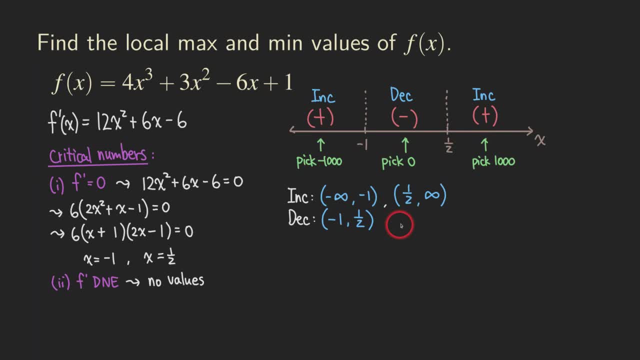 Okay, Now how do we find the local maximum and minimum points? Um, if we just try to imagine a little bit what the function looks like- and we can actually do a like a really rough sketch on the sign analysis chart to show it- 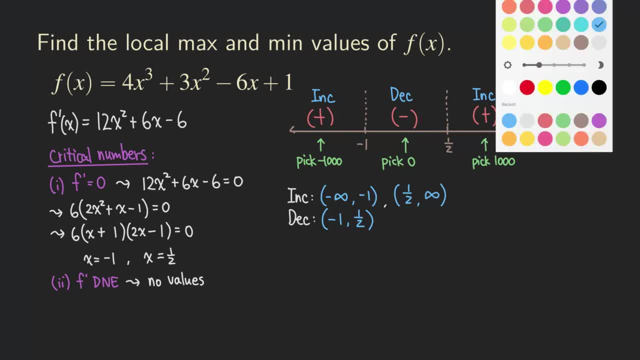 How do we show it? It's this: Now we know that the function has been increasing since like the infinity, and then it will change to um, decreasing when it goes past like the one right. So we know that it's going to be increasing. 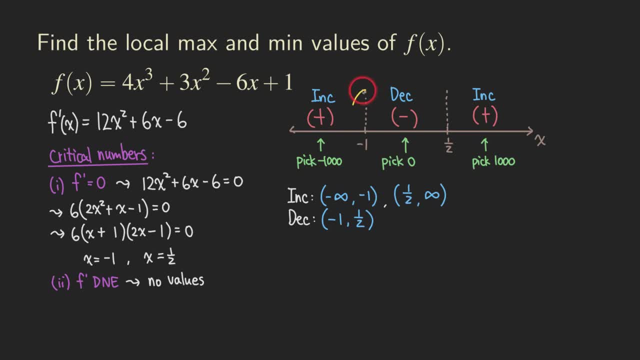 And then, once it hits this point, it will get a horizontal tangent. How do we know that it's the horizontal tangent? Because that's like the one- is the value that will make the um. Um. when we plug that into the first derivative, the first derivative will become zero. 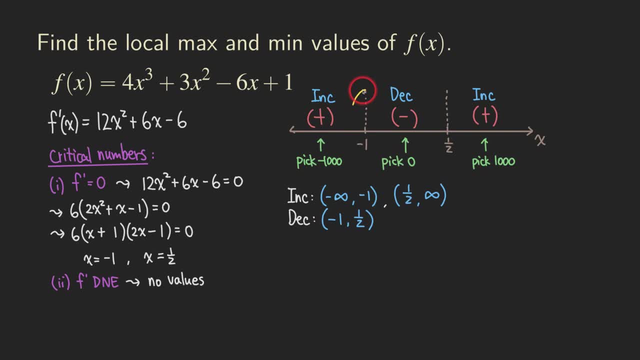 So we are getting a horizontal tangent here and then be um. beyond this point, then we are going to: uh, have a function, have the portion of the function that's decreasing. So it's going to go down with that, Okay. 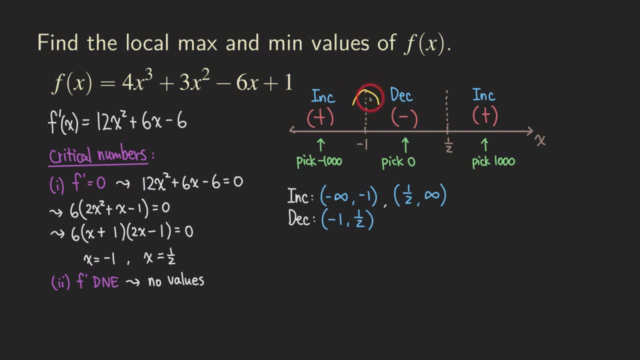 So now, as you can see here, we just look at this local area right here, Then we can see that that's actually a what a local maximum. Okay, Now, on the other hand, for the one half, we know that the function has been decreasing. 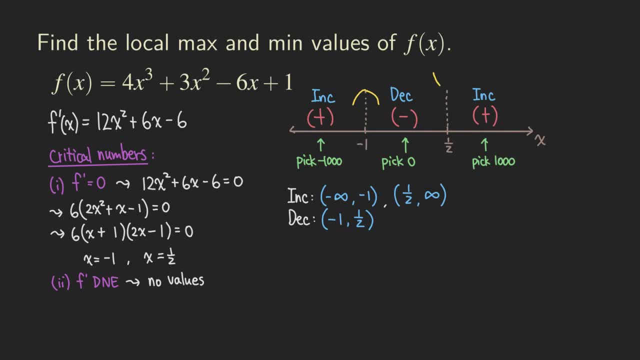 So we are going to get the um decreasing right here. And then do you see what's going on here? Once it passes the one half, it will turn into increasing right. So the function starts increasing after the one half. So you can see that that will be a local minimum. 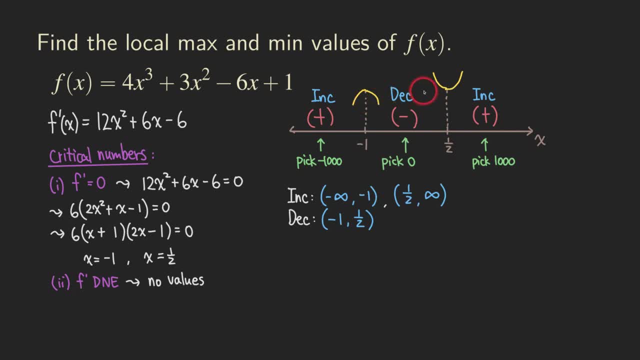 Okay, So we already have determined the maximum and the minimum And then? so now what do we do? We can just write down the result here. Okay, So here, um, for the local max value, right, or the local max value? 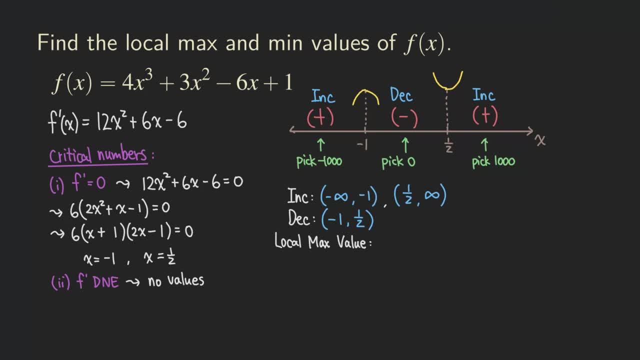 Oh yeah, So we have. how do we get that? We are going to plug in the- uh negative one into the original function because we're finding the Y value of the function. So we have F of With F, F of um. what is that? 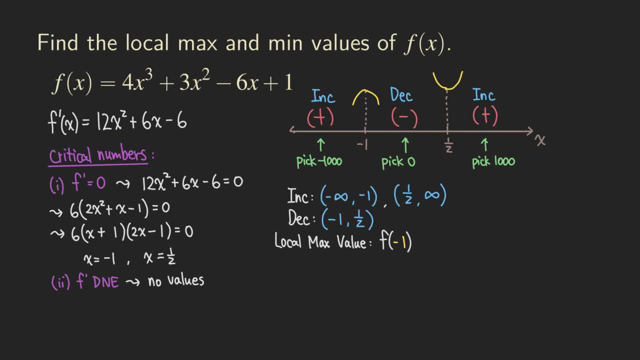 That's going to be a negative one in there. And then what do we get here? We are going to have four times something cubed plus square, minus six times something, and then plus one, And then all those Xs, all those blanks we are going to fill in the negative one. 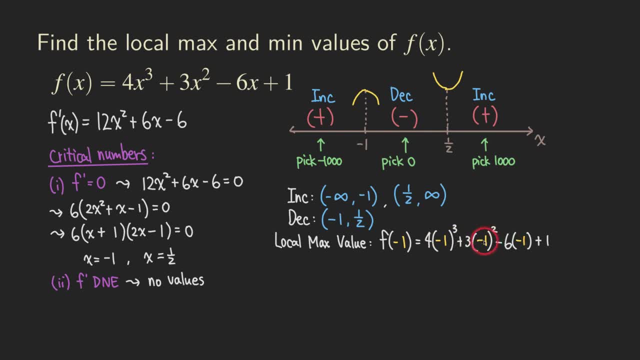 And then I'm not going to spend the time doing the calculation right here, I'm just going to, um, just write down the answer. The answer will be six. So the answer will be six for this one. and then, to just make it easier, 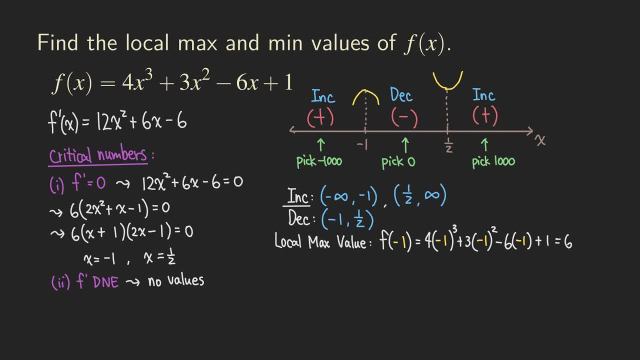 easier for us to read, right? So I'm going to just underline all those words right here. So now it's easier to read. And then, um, we also have a local minimum, right? So let's write it down as well. 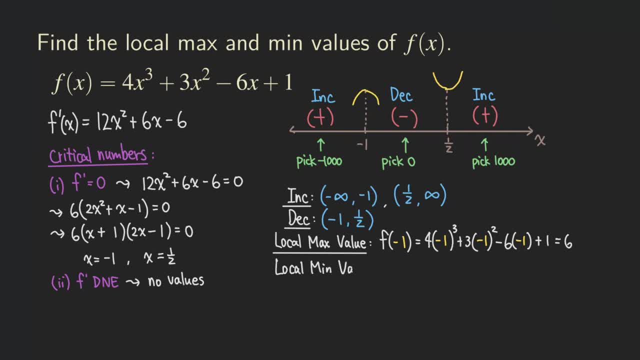 So we have our local minimum value, And let me just underline that. Okay, So what is the that value? So let's just write down the function first, Then we just fill that in. What is that? That's one half that we are going to plug in in there, right? 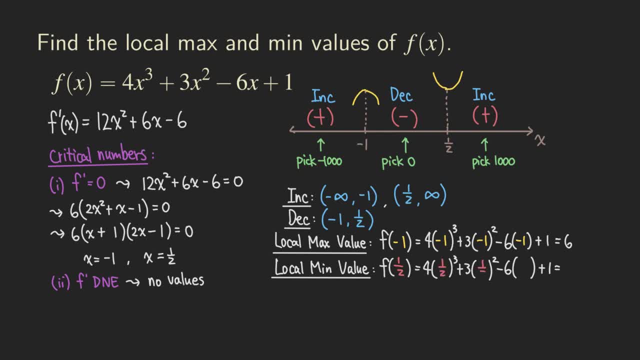 So we have one half one half and one half one half, and then you do all that calculation. Right, You can use your calculator or you can do it manually by hand, It doesn't really matter- And eventually we are going to get the answer to be a negative three over four.